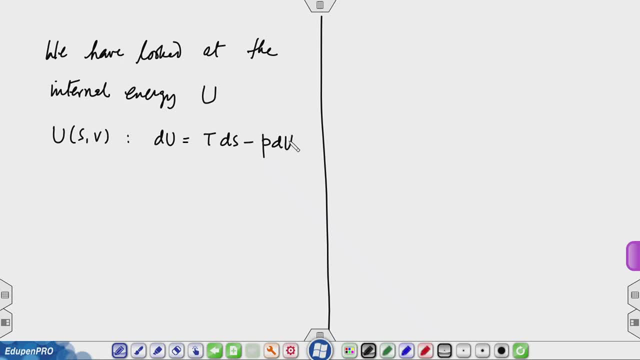 minus P dV, Or I should say from the central equation. and this is also equal to partial U with respect to partial V, or partial S at constant V times dS, plus partial U over partial V at constant S dV. And this gave partial U, partial S at constant S times dS, plus partial U over partial V at. 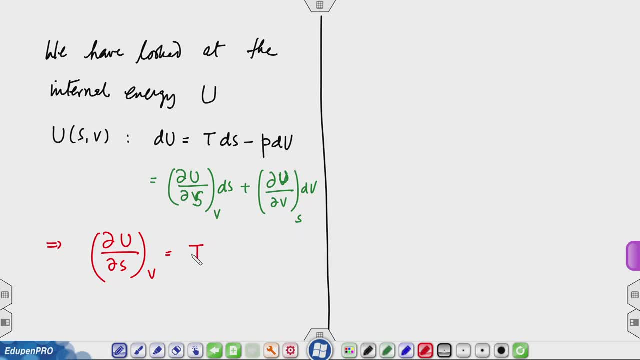 constant V, equal to the temperature, and partial U over partial V at constant S, V equal to minus the pressure, and this also led to Maxwell relation. Similarly, we define the enthalpy, which is another thermodynamic function, a potential, Where H was defined as U plus pressure times, volume, and d. H then came out to be T d S plus. 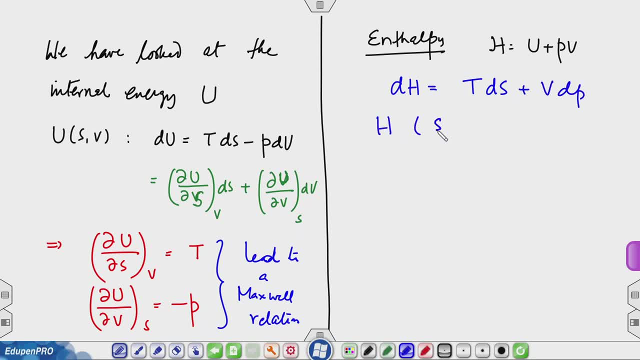 V d P, So H, the function of S and P. I can also write this, then, as equal to d H d S at constant pressure times, d S plus d H d P at constant entropy, d P. And that gave d H d S at constant pressure to be equal to T and d H d P at constant entropy to be equal. 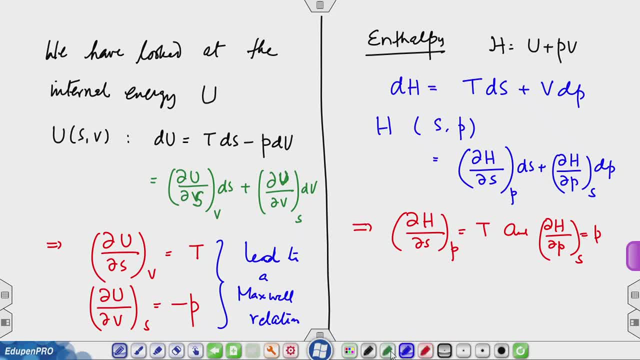 to P. So this is the case for the enthalpy case, and these processes become useful while describing constant volume or isochoric process in the case of internal energy and isobaric process in the case of enthalpy. What about if something else is a constant? suppose temperature is. 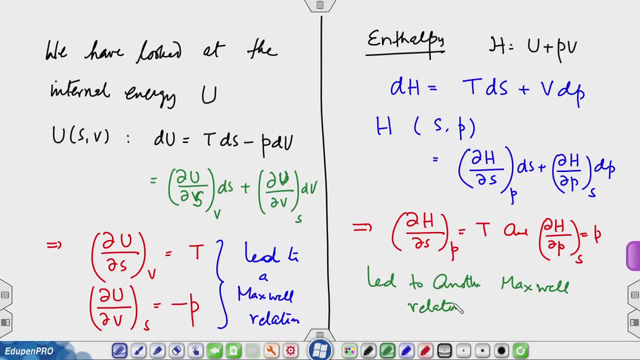 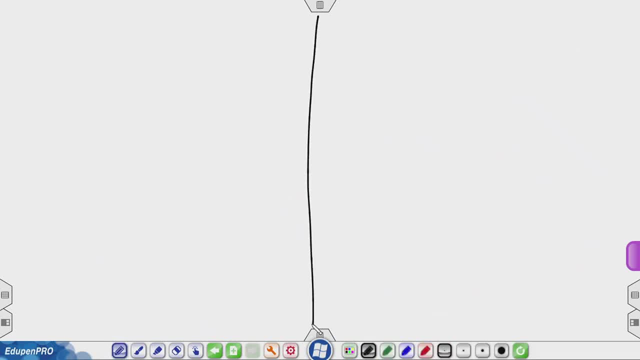 a constant volume is a constant. what happens then? In that case, we define another thermodynamic potential, and that is going to be the topic of discussion in this lecture. So here we are going to discuss another thermodynamic potential, known as the Helmholtz function, or 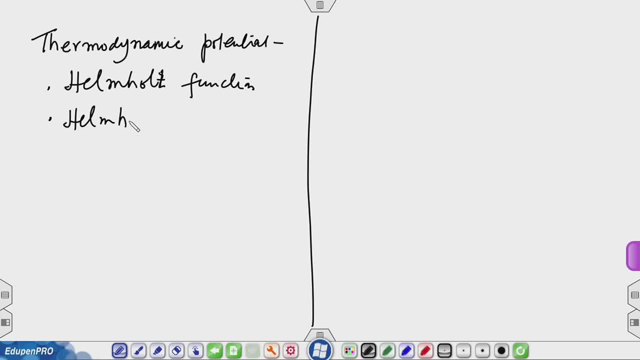 also Helmholtz free. 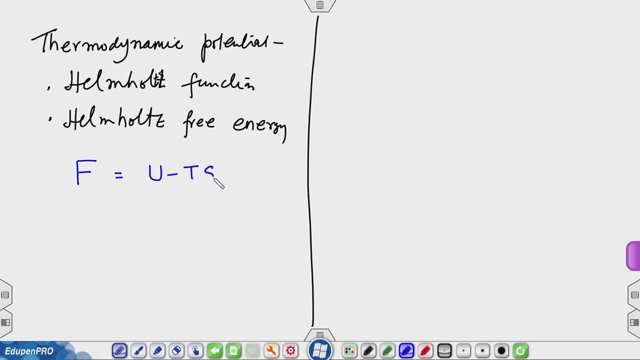 as U minus T S, and this implies that the differential D F is equal to D? U minus D T times S minus T D S and D? U can be written as T D S minus P, D V minus S D T minus T D S is anyway there. 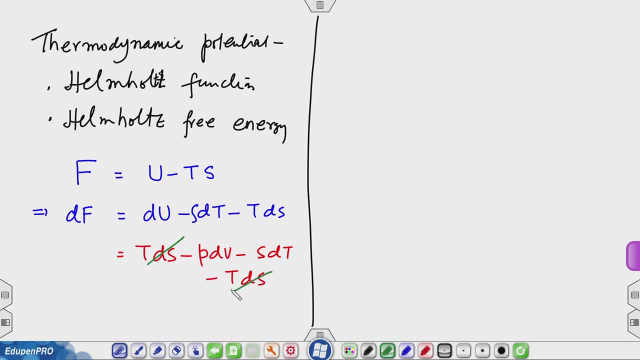 So T D S cancels and we get D. F is equal to minus P D V, minus S D T. So Helmholtz free energy F can be thought of as a function of V and T, and D. F, which is an exact or perfect differential, is equal to minus P D V, minus S D T. This is also equal. 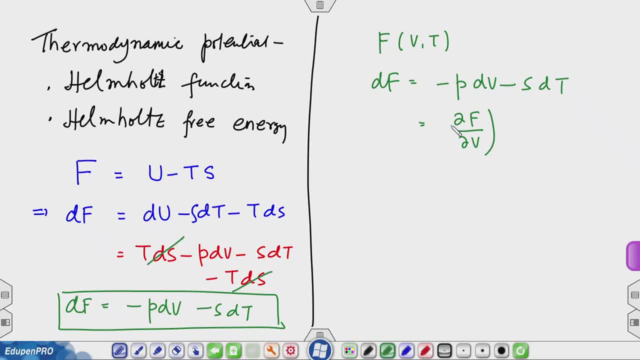 to partial of F with respect to partial V at constant temperature D V, plus partial derivative of F with respect to T at constant volume D T. and again, I remind you, this is an exact or a perfect differential And therefore from this I can derive another. 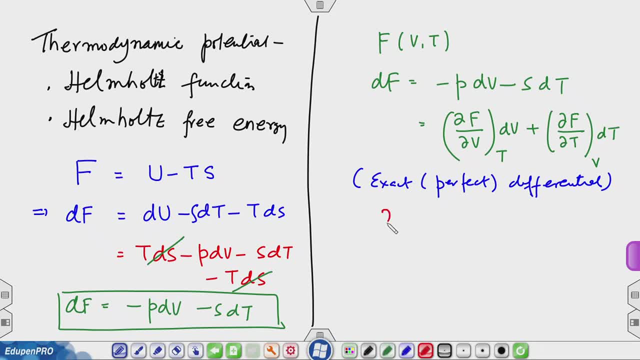 Maxwell relation. Now, from this we get partial F. partial V at constant temperature is equal to minus P and partial F, partial T at constant volume is equal to minus S. and since this is an exact differential, This leads to Maxwell relationship: partial P with respect to partial T at constant 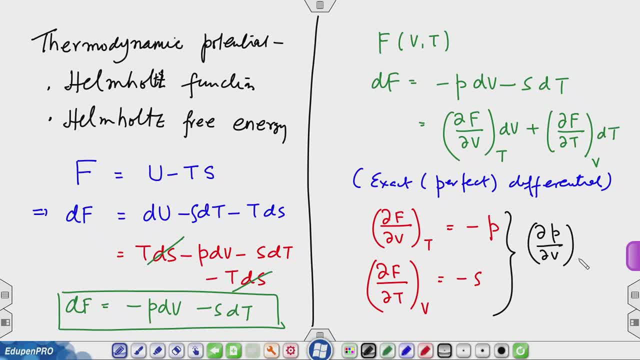 volume. partial v at constant partial v, p with respect to partial t at constant v will be equal to partial s with respect to partial v at constant t. This is the Maxwell relation. So let me just repeat this in the next slide. We have taken a thermodynamic 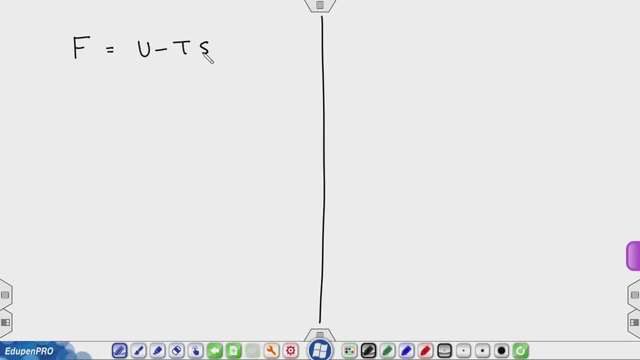 function f, which is u minus d s, and from this we have obtained that the differential, exact differential d f is equal to minus p d v, minus s d t, And equating this to partial f, partial v, at constant t d v plus partial f, partial. 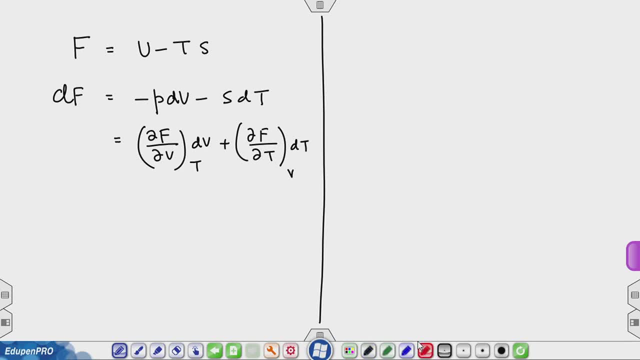 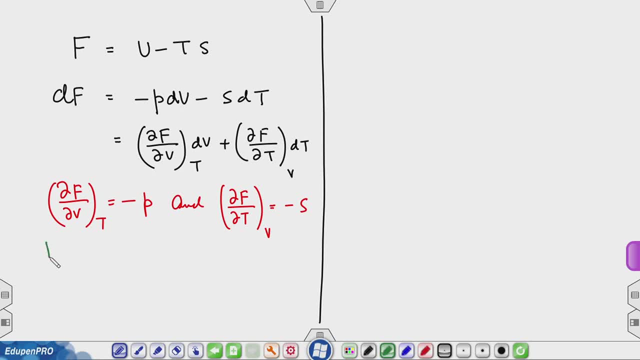 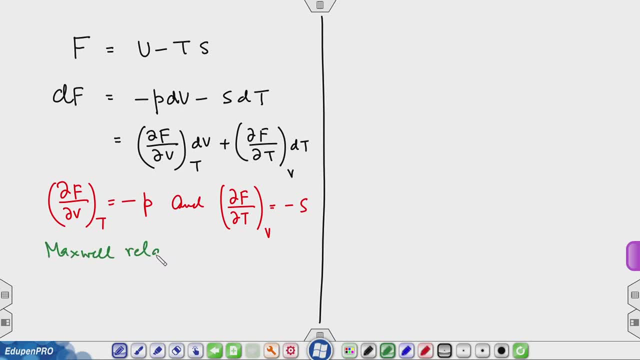 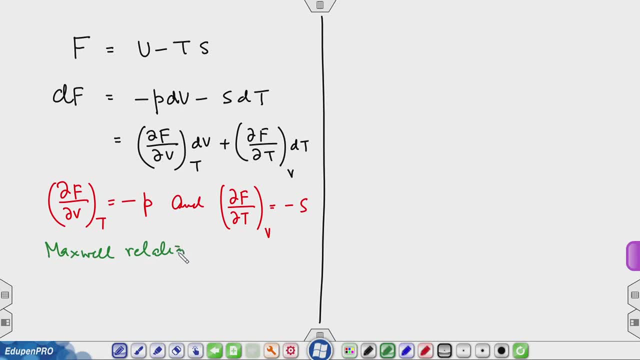 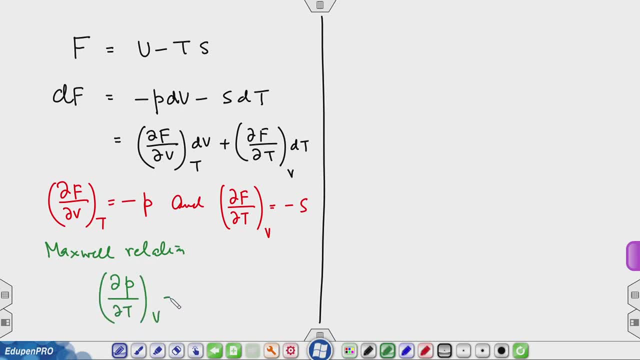 with respect to t at constant v is equal to partial s over partial v at constant t. That's the Maxwell relation. So you can see from these equations that Helmholtz function is going to be useful in describing processes that are isochoric. 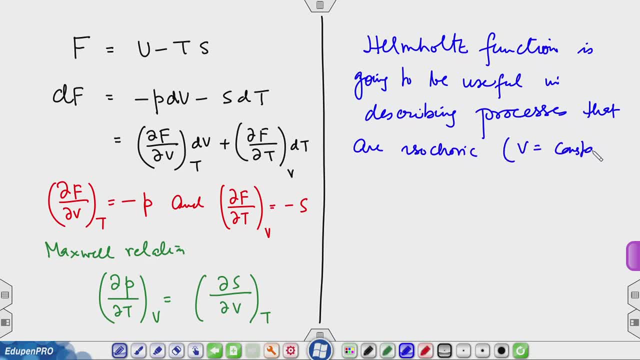 that is v equal to p, T equals constant and isothermal that is t equals constant. And we'll do that, but before that let's use the Maxwell relation derived to show two things. So first, I'm going to use the Maxwell relation obtained here to get two important results. 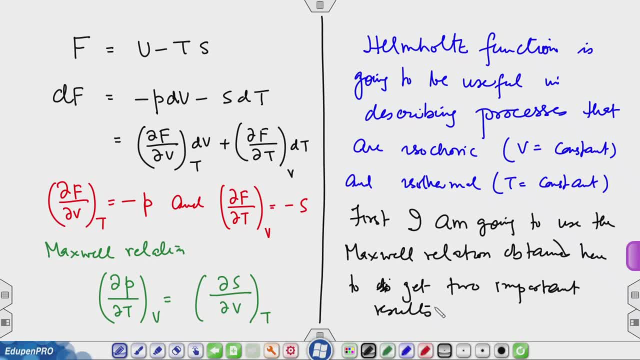 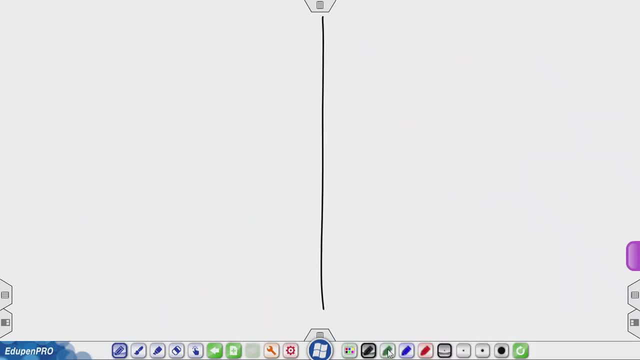 So let's do that. What is the Maxwell relation that we obtain from f? that says that dp by d, t at constant v is equal to ds, d t at constant ds, dv at constant t. So first I'm going to use this to show that for an ideal gas the internal energy depends. 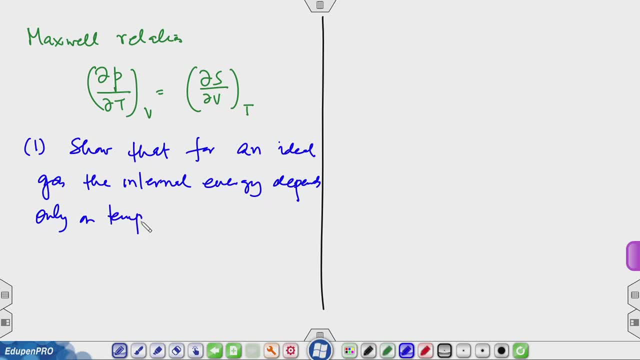 only on temperature. So to show this, if I can show that partial derivative of u with respect to v at constant temperature is 0, then we have proved it. Now recall from lectures in first week that I had said that u is a function of T only. So recall from lectures in first week that 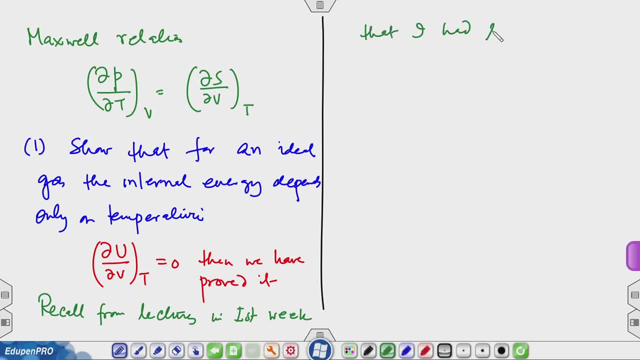 I had said: for an ideal gas, u is a function of T only, And also we had said that Rittman-Zemansky says that for an ideal gas, P, v equals n, R, T and u does not Depend on P. So we are now going to prove this. That time I had deferred the discussion. 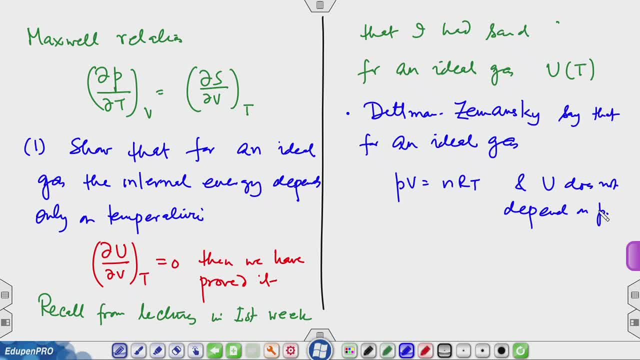 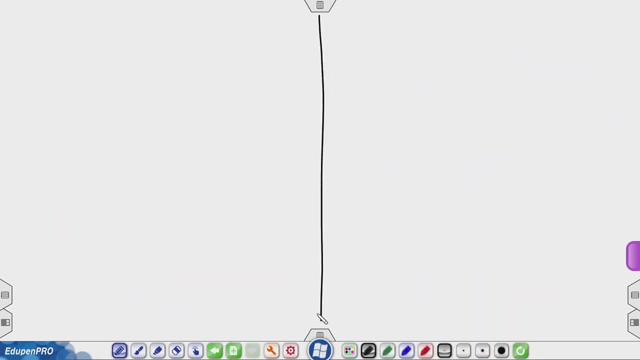 Now we are going to prove this using Maxwell relation and the equation of state. So here we prove this using the equation of state. for the ideal gas, P v, is a normal gas and the Maxwell relation obtained above. Let us do that. So if I take 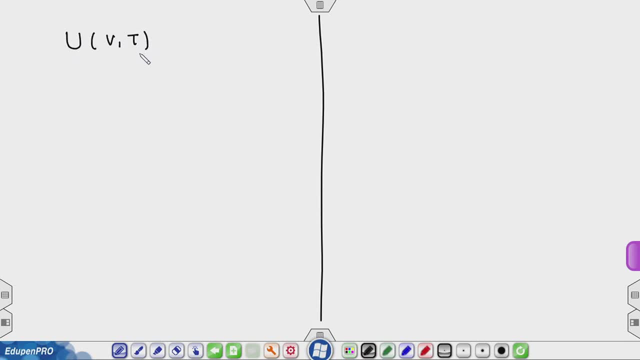 u as a function of v and T, then d? u is not a normal gas. If I take u as a function of T and v as a function of x, then this is not a normal gas, right? This is a normal gas. 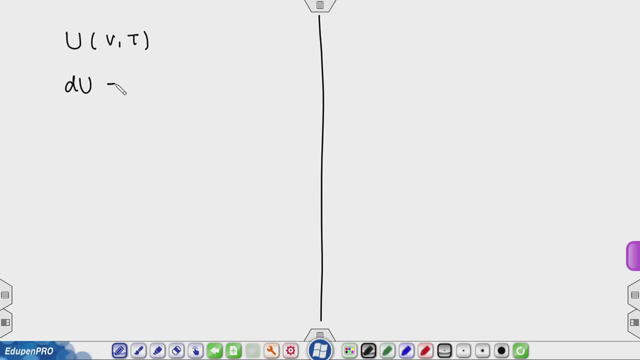 and I will remember that in a few times. Okay, Okay is sorry. u as a function of T n, s. I know d? u is T, d s minus P, d, v, And therefore partial derivative of u with respect to v. at a fixed temperature, T is going to be equal to T power. 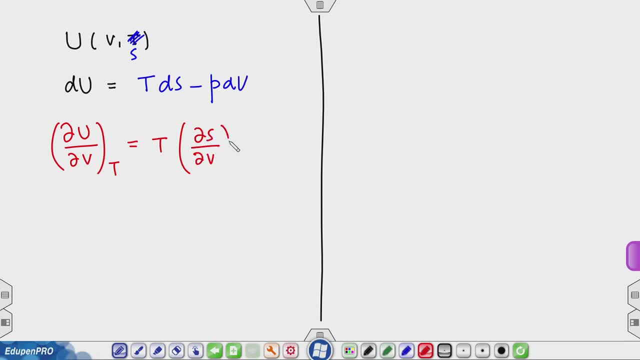 partial derivative of T with respect s with respect to v at fixed temperature, T minus P. Now I am going to use the Maxwell relation and write: d s by d v at T is equal to d s by d v at T. So d s is equal to d P by d T at v, And therefore partial u with respect to partial v at constant. 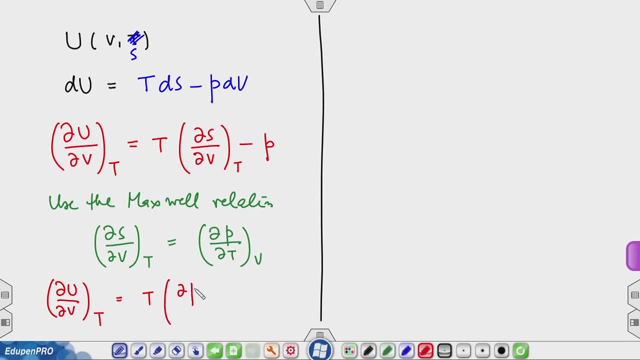 temperature is equal to T, d, P d, T at constant volume minus P. Now the equation of state for an ideal gas is P? v equals n r T. I can write P equals n r T over v And therefore partial P with respect to T at constant volume is going to be n? r over v And therefore 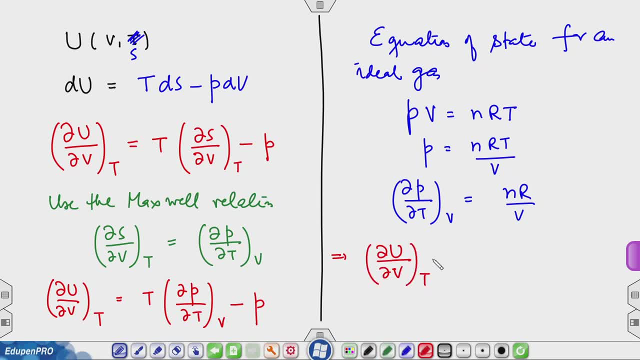 partial u with respect to T at constant temperature is going to be n r T this time around, Which is equal to n r T at this value 0.. Now this part on this fellow. So I am going to write n r T over v, So I am going to write n r T at opposite every times, And therefore 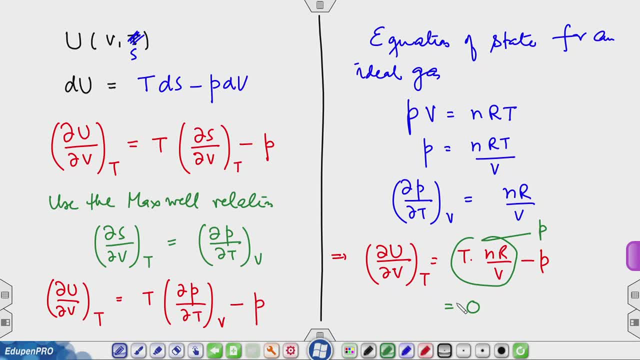 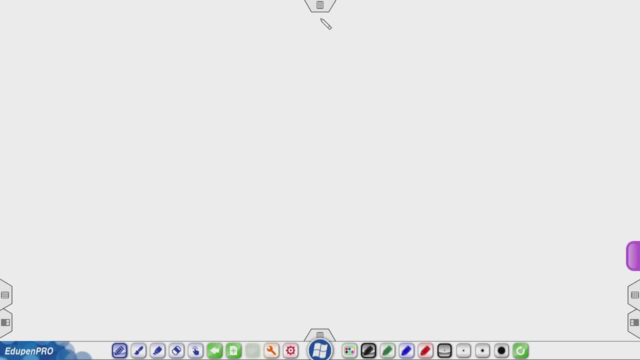 partial u with respect to T at constant temperature is equal to capital U with respect to T. Now for an ideal gas, the change in U, if I change its volume, keeping T constant, is 0 and this implies U does not depend on the volume of the ideal gas or U depends only on the temperature. 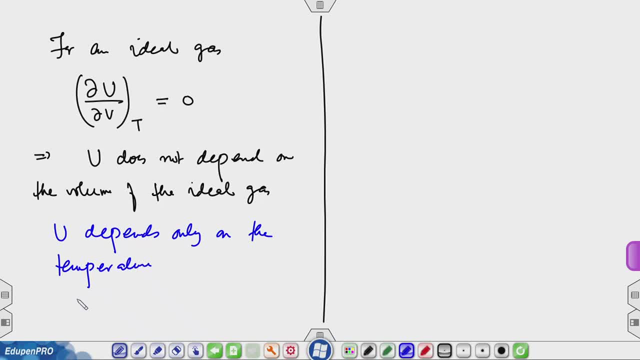 So if I consider U as a function of V and T will be equal to U of T, only Using the same, extending it further. using the same argument, I can also show that if I write U as a function of P and T, this is also P equal to U and T. why? because, if I 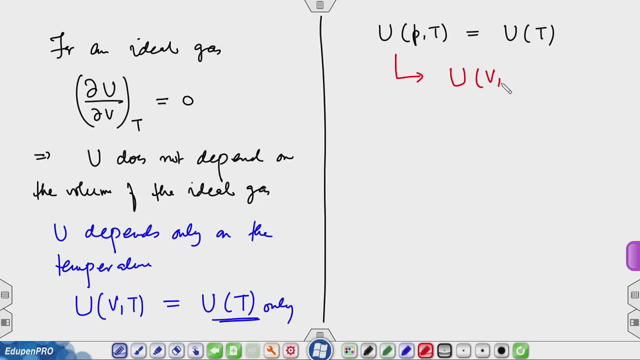 take U, P and T. I can write this as U, V and T, So I am using the equation of state and U V, T is U, T alone. So U does not depend on P also, Because if it did, then the dependence on V will also come in the lecture on another. 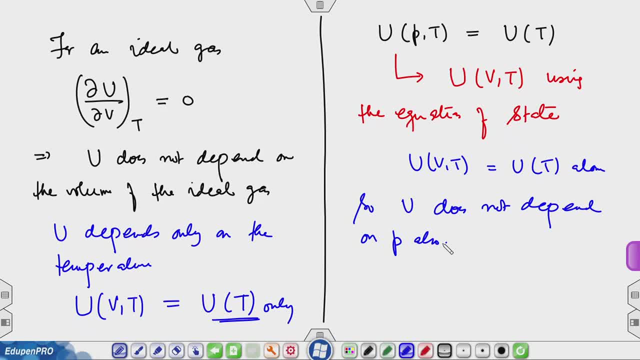 thermodynamic potential called Gibbs free energy. We will prove this explicitly because I will get a Maxwell relation there relating the pressure partial derivative. So that is one result based on the Maxwell relation. The second result I am going to obtain is is Stefan Boltzmann law for black body radiation. so let me just recall first, 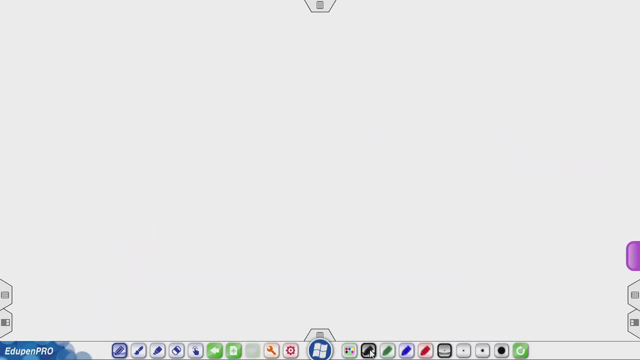 what black body radiation is, or Stefan Boltzmann law is all about. if I take a black body, that is a cavity where radiation is trapped, and let it come out from a hole, then the intensity of radiation is proportional to t raise to 4 and you can also show that. 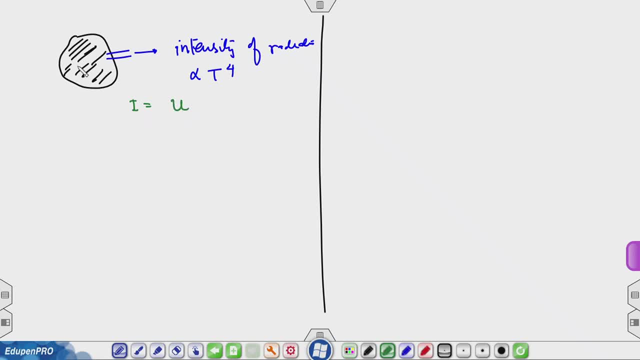 this intensity is equal to the energy density inside, which depends only on t c by 4, where c is the speed of light. now, experimentally, Stefan established that i is proportional to t raise to 4 and therefore this implies u t is also proportional to t raise to 4, or u t is some constant times t raise to 4. 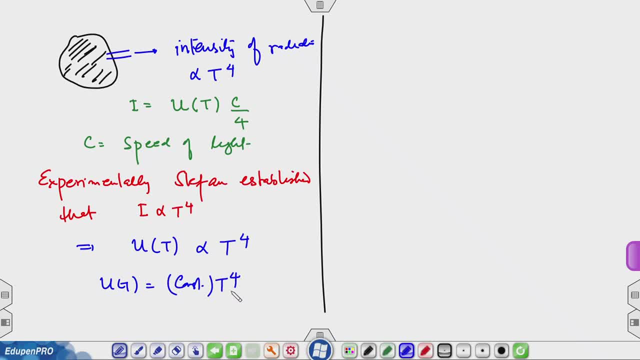 so this is known as Stefan Boltzmann law. now, where does the name Boltzmann come in? from that comes because now I am going to derive it theoretically using thermodynamics. so this is- this is experimental fact. now, theoretical equation of u t proportional to t, raise to 4 using thermodynamics. for this I need you. 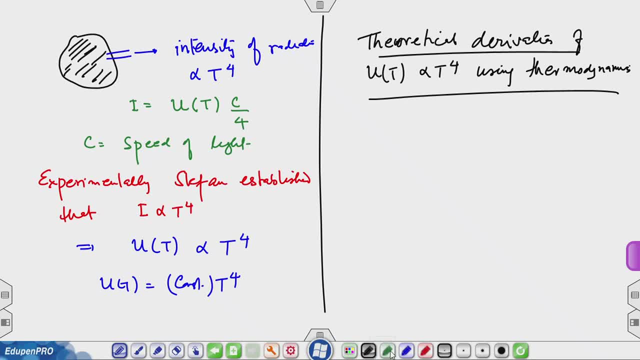 to know the following two things. suppose I have a this cavity and this is radiation going in here which is known as diffused radiation. this is diffused radiation because going all over the place that there is no plane wave kind of thing is diffused, in this case the radiation. 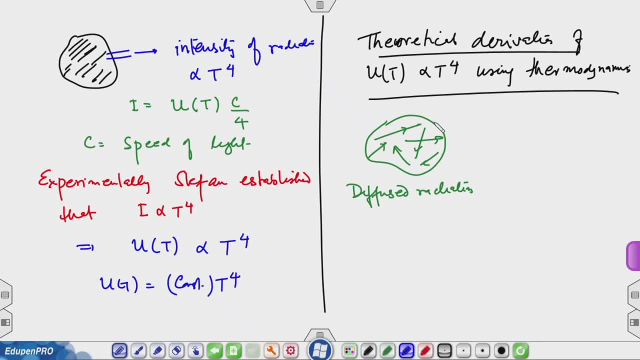 also gives pressure on the walls. so if this has intensity u, t, then the pressure p due to this radiation, is also a function of t only and it is u by 3, and this is known. that the, the internal energy or the pressure, depends only on temperature, that is known, it does. 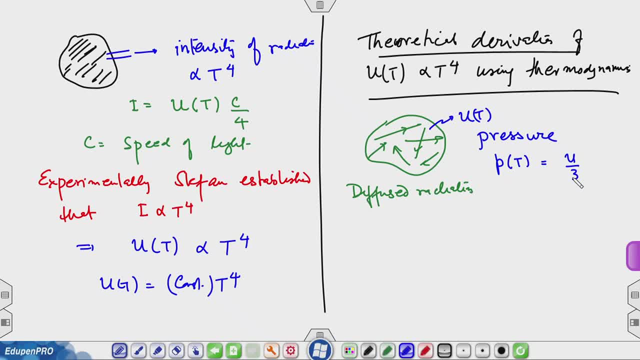 not depend on the volume, only on temperature. so we are now going to use this fact. now, use d? u equals t, d s minus t, raise to 4. p d v and write: partial u with respect to partial v at constant temperature is equal to t, partial s, partial v at constant temperature minus p. so this is exactly what we are doing. 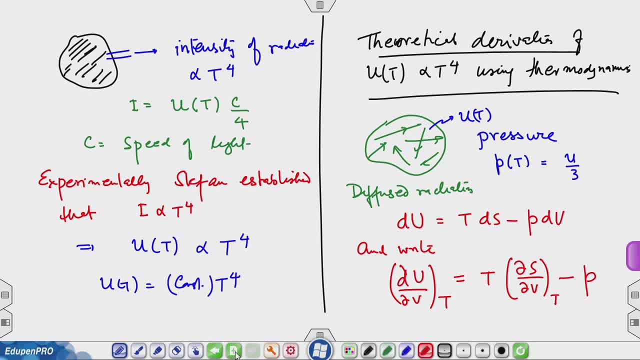 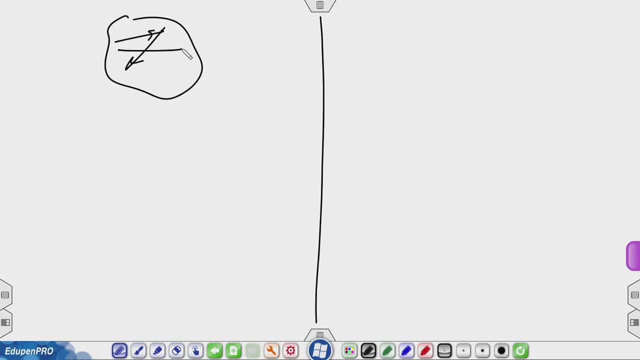 in the case of ideal gas. Now we are applying. Now we are applying – P, P u. partial v at constant temperature is equal to T. partial s, partial v at constant temperature minus p. I use the Maxwell relation. partial s over partial v at constant T is equal to. 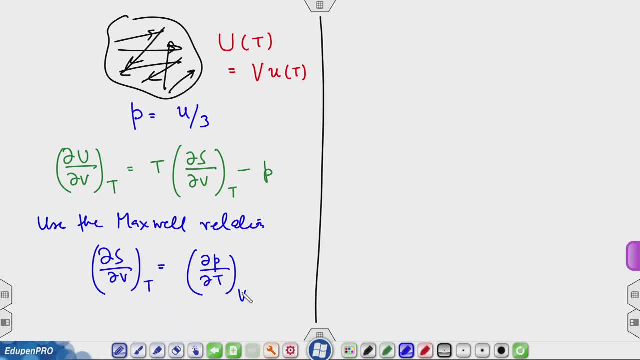 partial p over partial T at constant v, And then we get d by d v of u. v at constant temperature is equal to T, d p. d T at constant v minus p, Since the small u depends only on the temperature on the left hand side, I get d: v at constant temperature minus p. 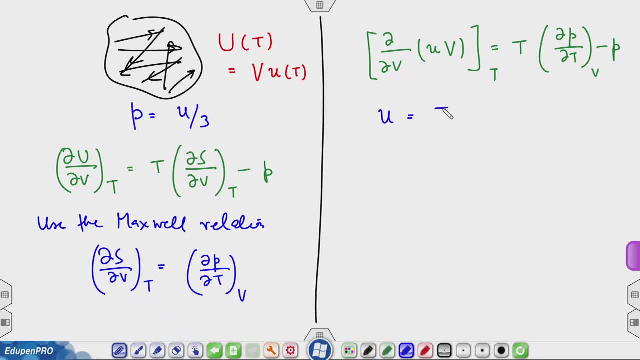 Since the small u depends only on the temperature. on the left hand side I get d, v at constant temperature, plus u, which is equal to T, and for p I use u by 3.. So this gets T by 3, d, u, d, T at constant volume. so, given a volume, that is what I get, minus u by 3.. And this 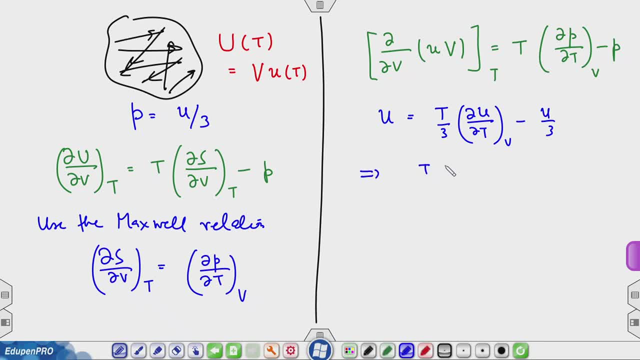 gives you T d, u by d, T at constant volume is equal to 4 u, And that immediately implies that u t is proportional to t raise to 4.. So, experimentally, Stefan establishes that u is proportional to t raise to 4, you know all this law, you. 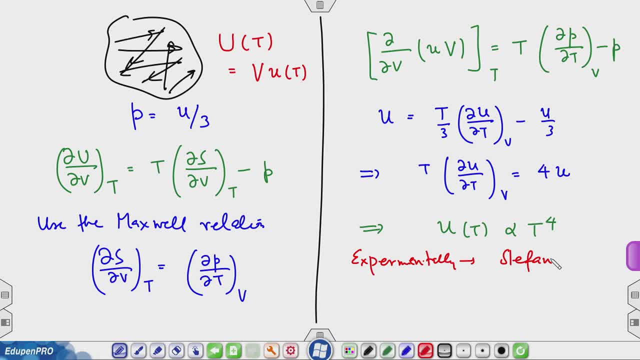 have been using in your twelfth grade. sigma t raise to 4 is the intensity and, theoretically, Boltzmann, who gives this law on the basis of thermodynamics. So this is known as Stefan Boltzmann law: that intensity sigma t raise to 4.. 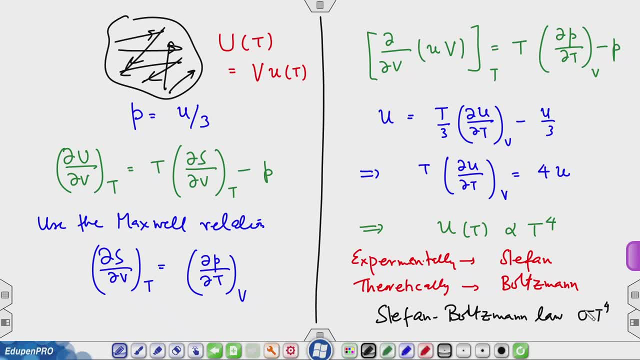 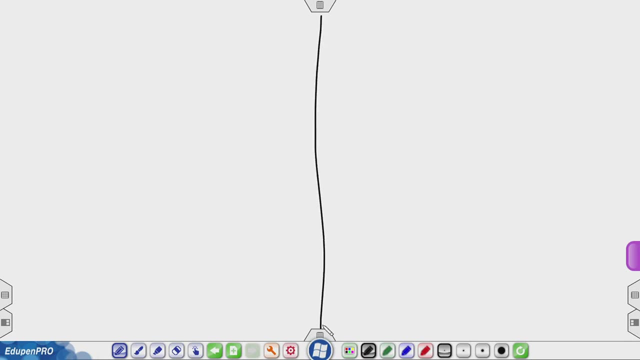 So this is an application of the Maxwell relation. Now let us discuss further significance of Helmholtz free energy. So you have done the Maxwell relations through whatever we obtain through the Helmholtz free energy. now we want to discuss this further significance. 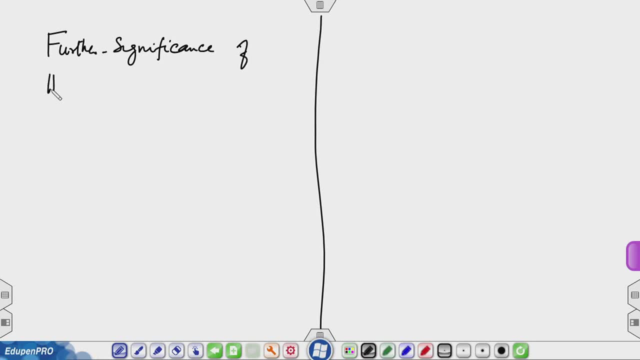 So this: right now we will Consider systems that are in touch with a reservoir. it is a heat reservoir at temperature. 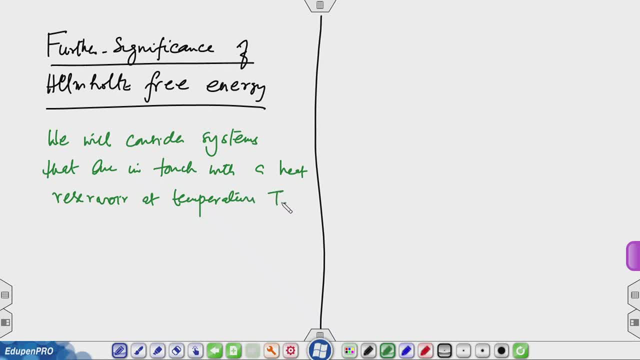 T. So first, what we want to show is that if the system is in a non-equilibrium state and goes towards equilibrium, then delta F is less than equal to 0.. You may say: if there is a non-equilibrium state, why is it that we are thinking that it can have a state function like F? So what we 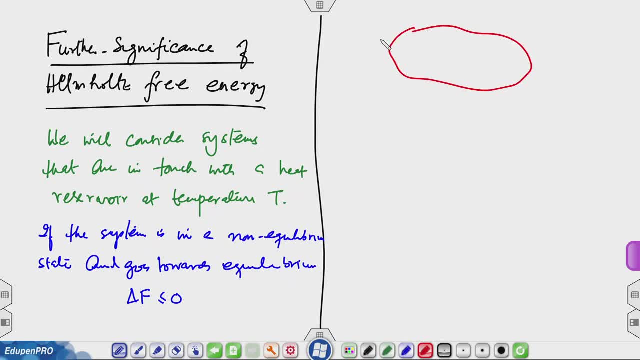 can say: is suppose there is a system which is in non-equilibrium state. I can divide this into small, small systems, considering each one to be in equilibrium and then write: F equals summation, delta F over each, And considering that the gradient of whatever properties are inside they are not strong. 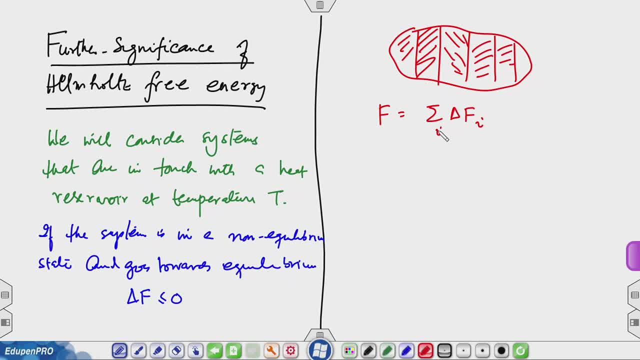 enough that they do not contribute. the gradients do not contribute to the free energy. only the value of those properties, V or T or whatever- in these small sections gives the free energy. So that is how one can think of this. So if a system is changing spontaneously, it 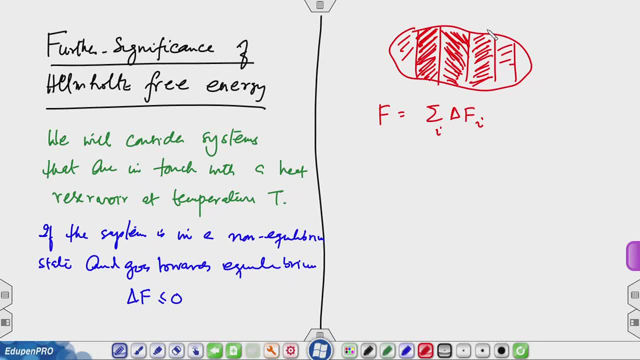 it is going towards equilibrium. this is what happens. Let us show this and this I point out now and I will keep pointing it out: this is a result of entropene fees of universe. So the system, the universe we are considering is there is this heat reservoir and inside 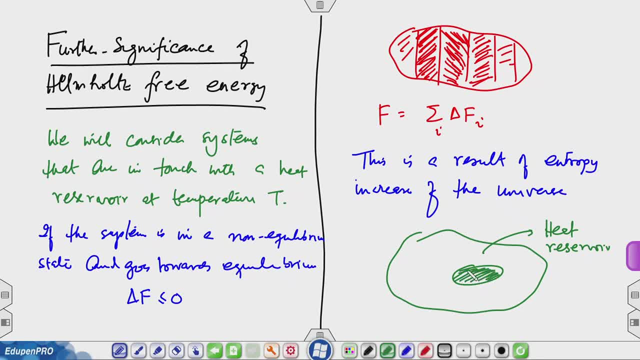 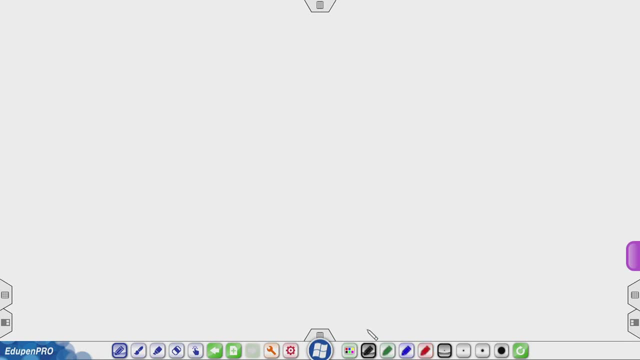 there is some system and the two can exchange heat. So we will now consider, take the system to be at constant volume. It is under these conditions that delta f will be less than equal to 0. volume of the system is constant then, as number 1 to Q given by the reservoir to the system. 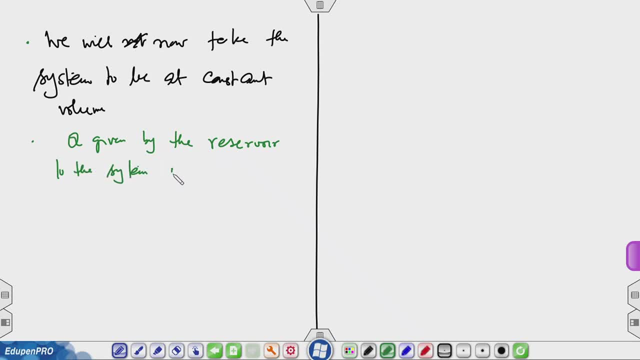 will be equal to the internal energy change delta U of the system. And third, delta S will be equal to delta S reservoir Plus delta S system. since heat is being given away by the reservoir, this is going to be minus Q and reservoir is at fixed temperature: T plus delta S. Now I am dropping the system. 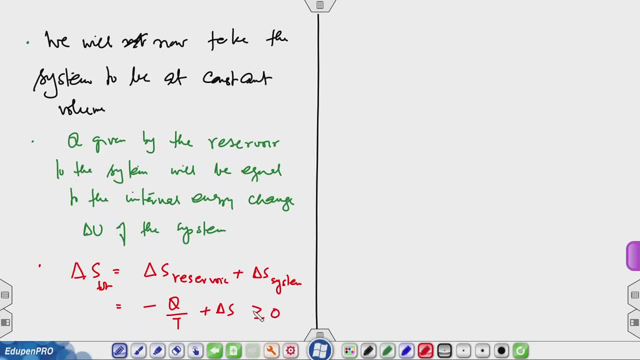 and this should be greater than or equal to 0.. So what do we have? We have, minus Q, plus T, delta S is greater than or equal to 0.. Now Q is equal to delta U system. 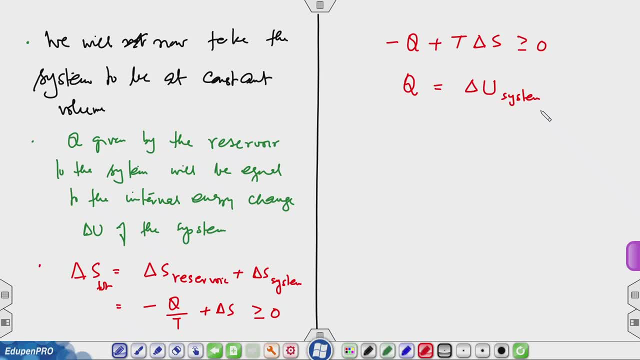 entropy increase of the universe, Nothing else. and this is expressed. delta s is expressed. 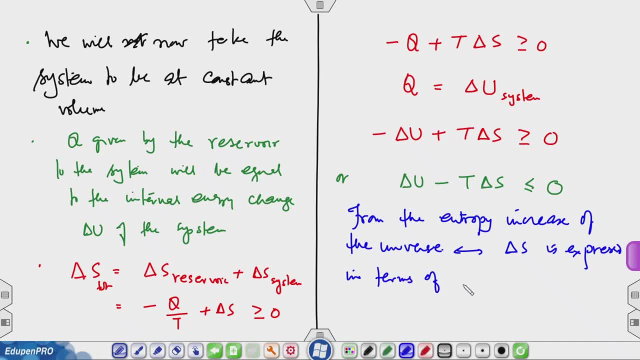 in terms of the system properties. That is all we are doing. although we are writing this in terms of system properties, you have to keep in mind that what we are finally doing is that the entropy of the universe is being taken to be increasing, and that is the sum. 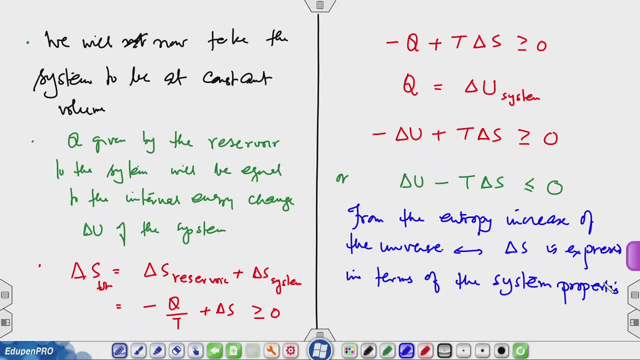 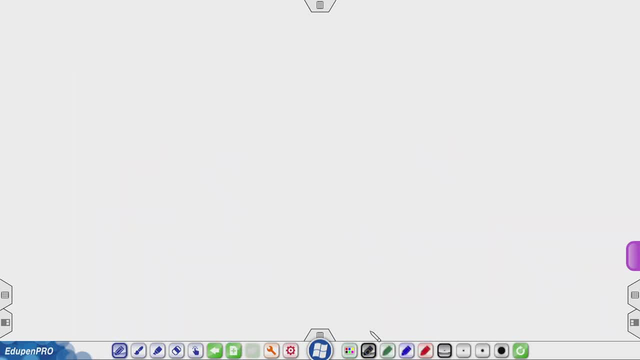 of the entropy change of the reservoir, plus and the plus the entropy change of the system. So now, since t is fixed, this gives you delta u minus t. delta s equals. delta of u minus t s should be less than equal to 0, and this is nothing, but this implies delta f is less. 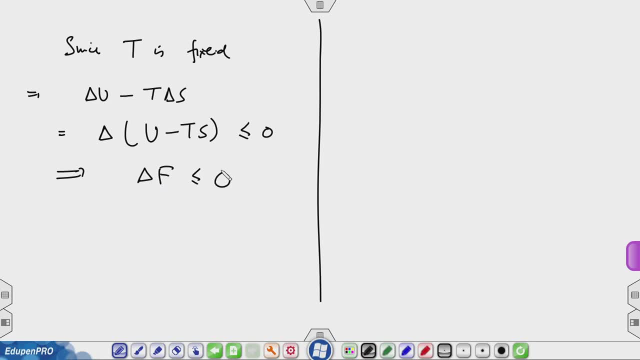 than equal to 0.. Now remark: since v is fixed, that is why we took q to be equal to minus delta or plus delta. u And t at the end points of the process is fixed. delta f less than equal to 0 is independent. 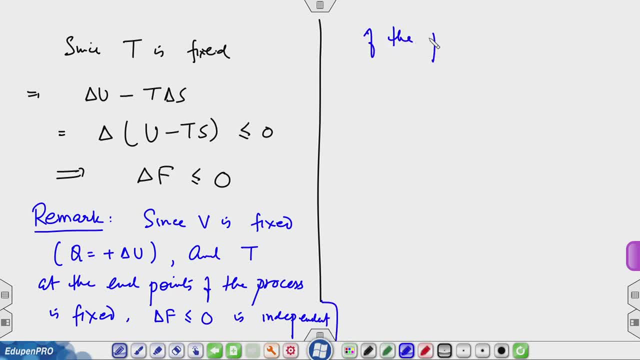 of the process going from one state to the other. What it means is that, since f is a state function And it is being evaluated at v and t at the end of two processes- So that is what it is- delta f will tend to lower value. Now, as equilibrium is reached, then system does. 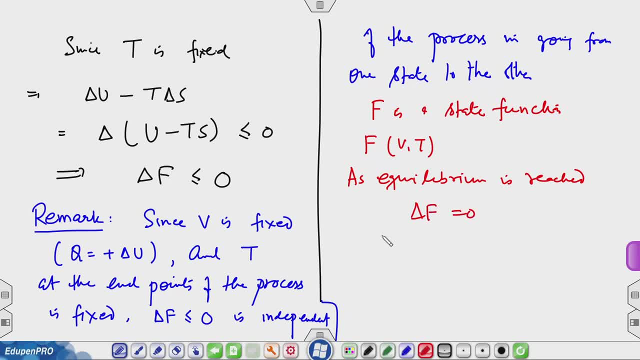 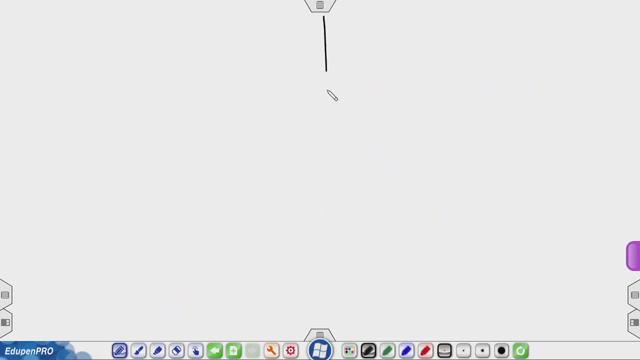 not change any longer And delta f will be 0. And delta f attains its minimum value. So we can conclude as a system undergoes or spontaneous process or change at constant volume And is in contact with the heat reservoir at temperature T. 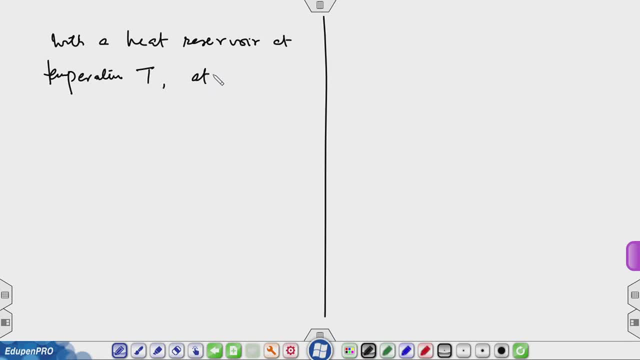 And at temperature T And at temperature T At few value as it attain equilibrium, F takes minimum value. Now notice how we calculated F. if delta F is calculated as delta U minus T, delta S, which is delta U minus T minus t, delta s, the t at the beginning and at the end of the process is the same In. 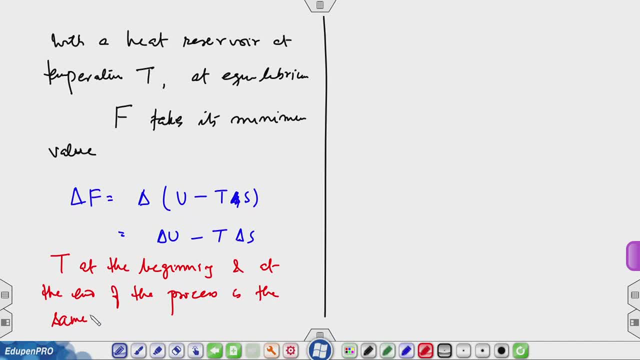 between there could be changes, but right at the beginning and at the end, t is the same. This is very important when we discuss the next significance of the Helmholtz free energy, and that is, it gives you the maximum possible work that a system can do. Now, here, before. 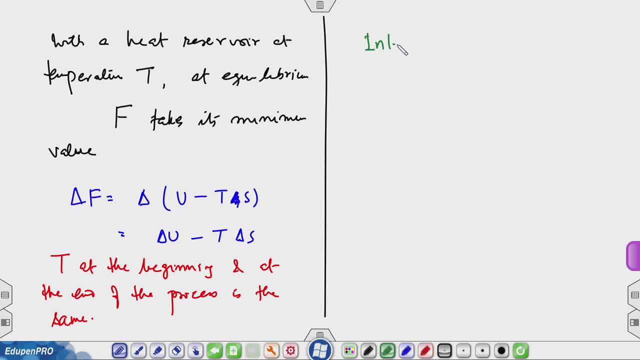 we do that. I want to discuss an interpretation, Pointing out wrong one and the correct one. When you look at, delta F equals delta u minus t, delta s is less than equal to 0. Then, as the system goes towards equilibrium, then an interpretation may be given, that an approach. 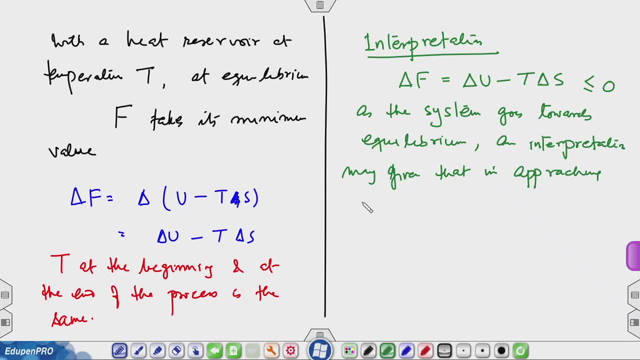 in equilibrium system lowers is internal energy u, So that delta u is less than 0, and increases So that delta s is greater than 0 and minus t, delta s is less than 0. But this is not correct. This is not correct because delta u is coming from the heat given by the reservoir. 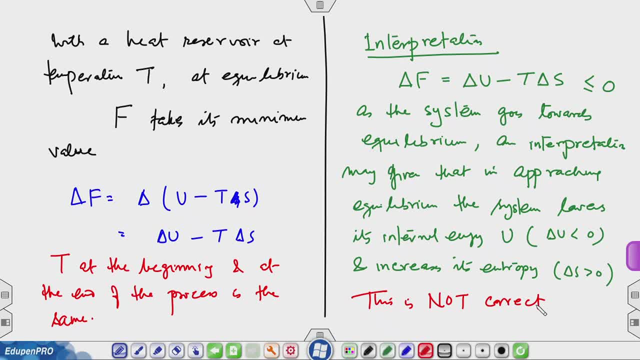 to the system and we are writing that in terms of the change of the internal energy of the system, The only, the only thing that is driving the system towards equilibrium, The only thing that is driving the system towards equilibrium, is the maximization of the entropy. S max drives system towards equilibrium. So keep this in mind and we can discuss it. 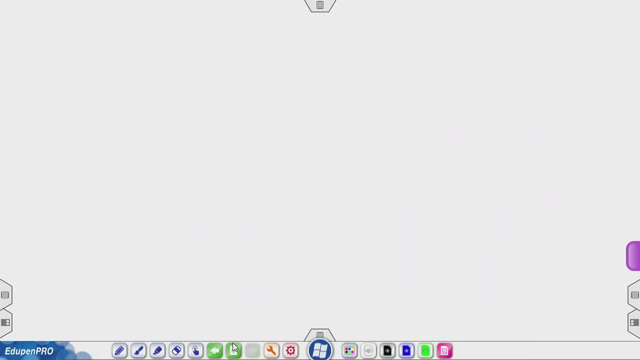 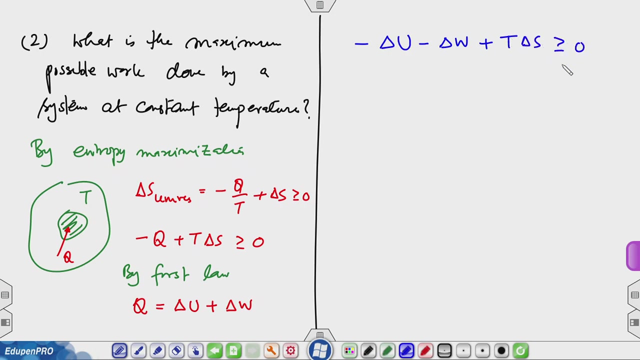 further in our tutorial Now. second significance of Helmholtz free energy is: what is the maximum possible work done by a system? 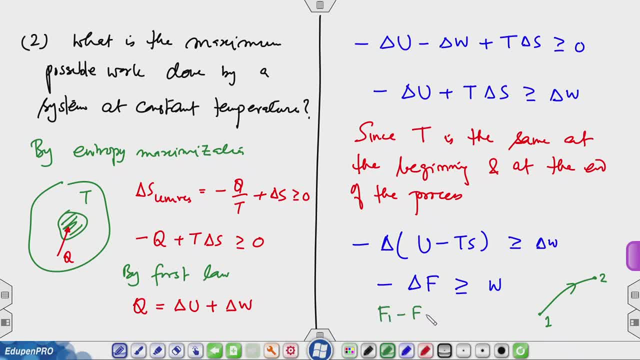 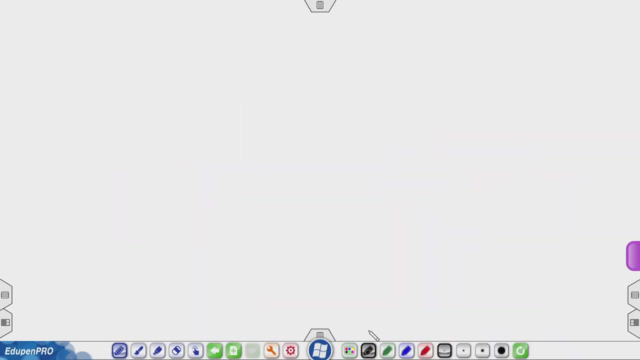 is the change in the internal energy of the system. Now this is slightly different from the mechanical systems. So in purely mechanical systems the work done will be equal to delta U. So work done will be given by the change in the internal energy of the system. 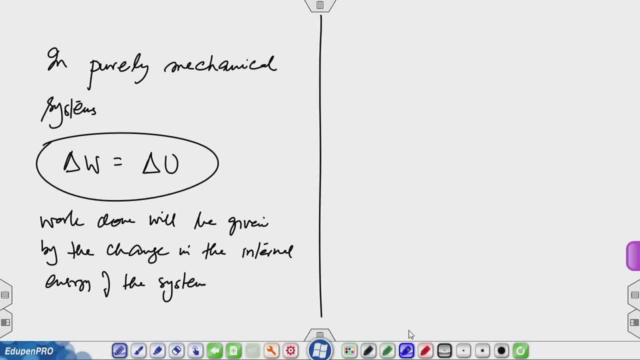 But what we have now is that U1 minus U2 plus T? S1 minus S2 is greater than or equal to W. Let's see if it is consistent. I have F, which is T? U minus T S, So F1 minus F2 will be equal to U1 minus U2, minus T S1 minus S2.. 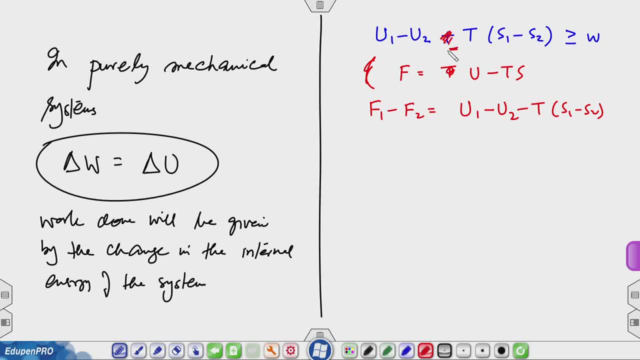 So this is minus. Now what is happening is, since there is heat exchange with the reservoir, that also contributes to the work done by the system. So suppose S1 is greater than S2.. This will imply some heat has gone to the reservoir and that means the work done will. 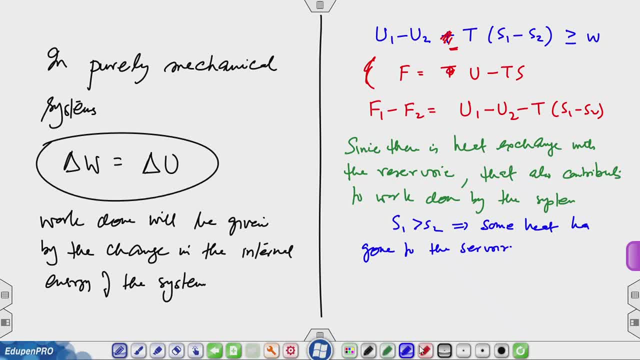 be less than U1 minus U2.. And if S1 is less than S2, this will imply some heat has entered the system from the reservoir and that will contribute to more work. So the thermodynamic system also takes care of you know the. 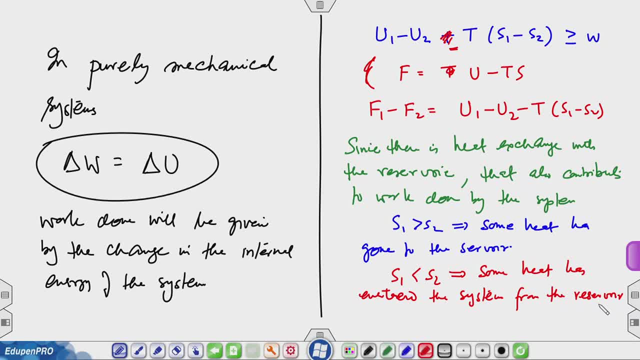 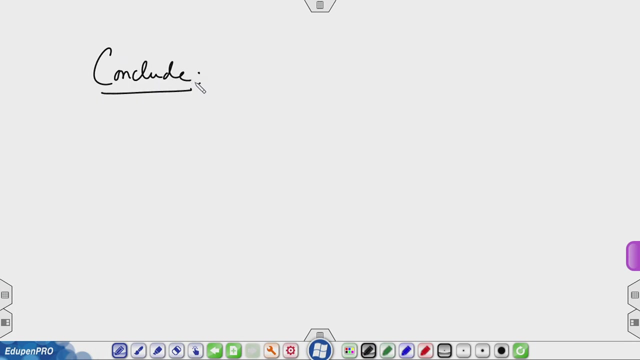 entropy change takes care of that heat exchange also. So it is the energy difference plus the heat that it is getting or giving to reservoir that limits or that determines the work done by the system. So with this let me now conclude this lecture, saying that 1 A nu. 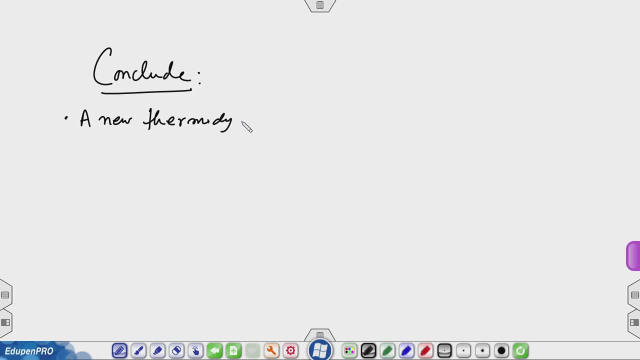 Thermodynamic potential, namely the Helmholtz function or Helmholtz free energy, has been reduced to using the corresponding Maxwell relation. We have shown that for an ideal gas U T, V is only U T, and also obtained Stefan-Boltzmann law. 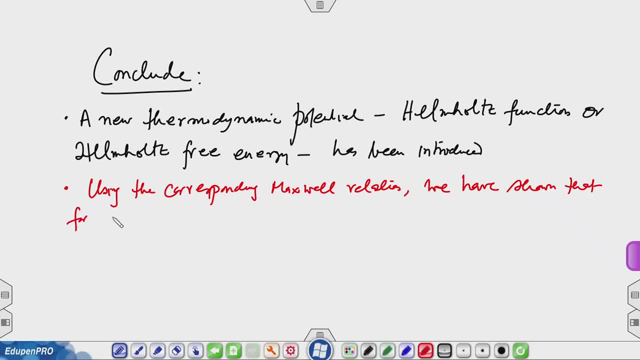 We have shown that for an ideal gas, U T V is only U? T and also obtained. Stefan-Boltzmann law Is simply of some kind of in P Constitution. in efficient minimum value and finally f delta f gives the maximum work done by a system. 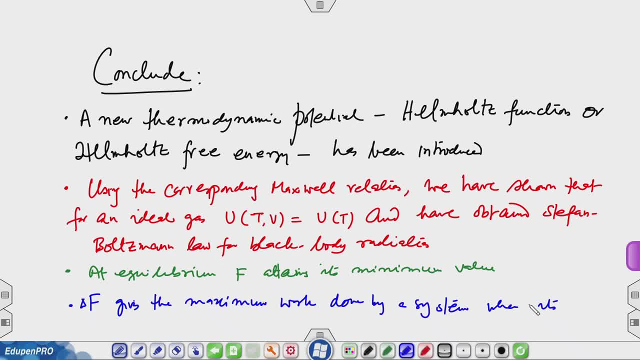 when its temperature at the beginning and end of the process are the same. Now the third point, which is written in green at equilibrium f attains its minimum value when the system is at constant volume and in touch with a heat reservoir. It should be not in touching contact. 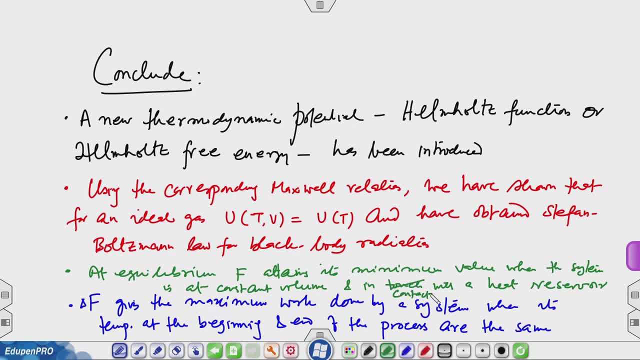 So we defined a new thermodynamic potential, Helmholtz function. Use the corresponding Maxwell relations to show that the internal energy of an ideal gas depends only on its temperature at equilibrium f attains as minimum value. So when the system is approaching equilibrium f becomes smaller and smaller and attains its minimum value. 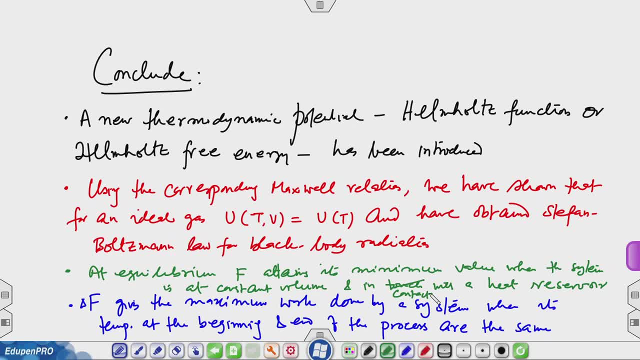 when the system is at. So the system being considered as a constant volume and in touch with a heat reservoir, at temperature t, then it attains f, attains its minimum value, But And delta F between two states gives the maximum work done by a system when its temperature at the beginning.